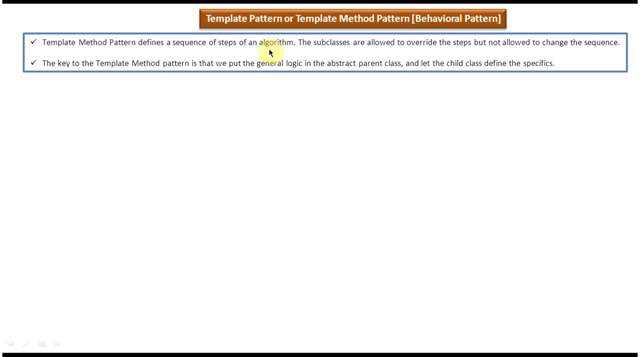 Hi, this video tutorial I will cover template design pattern. This template design pattern also called template method design pattern, and this template method design pattern falls under the category of behavioral pattern. First we will see the explanation of template method design pattern. This is the first explanation. I will just read out. 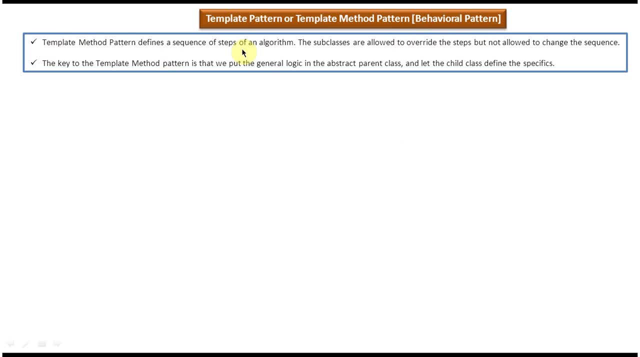 Template method pattern defines a sequence of steps of an algorithm. The subclass is allowed to overwrite the steps, but not allowed to change the sequence. This is the second explanation. The key to the template method design pattern is that we put the generic logic in the abstract parent class and let the child class define the specifics. 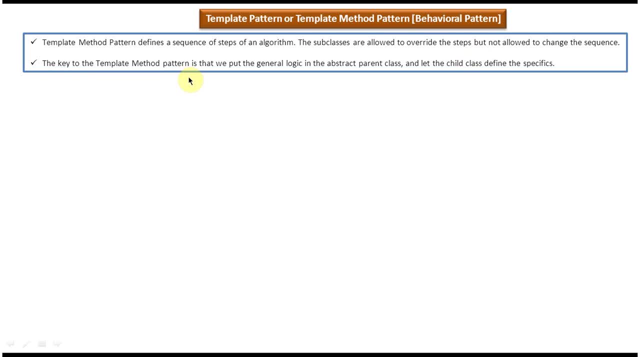 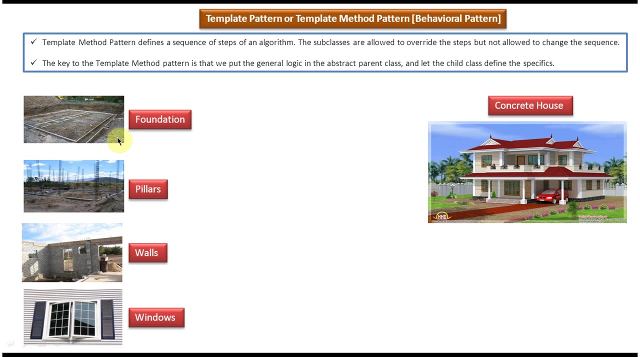 This is the explanation. We will see one example so that you will understand. understand this explanation very clearly. suppose, say, I want to build a concrete house, then what I have to do is, first, I have to build a foundation and second, I have to build a pillars. third, I have to. 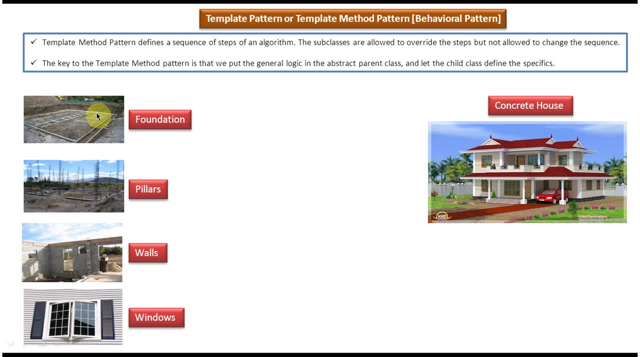 build a walls. fourth, I have to build a windows. so I have to follow this sequence of procedures in order to build a concrete house. right? suppose, say, I want to build a wooden house. so if I want to build a wooden house, I have to follow the same procedure which I followed in the concrete house, right? 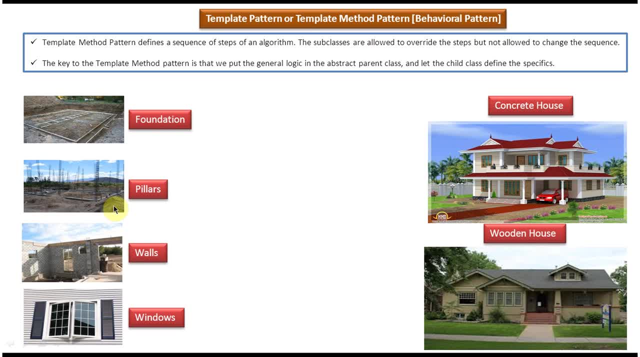 first I have to build a foundation, then I have to build a pillars, then I have to build a walls, then I have to build a windows. only difference is: instead of concrete, use wooden materials to build a wooden house. right, okay, so what I can do is I. 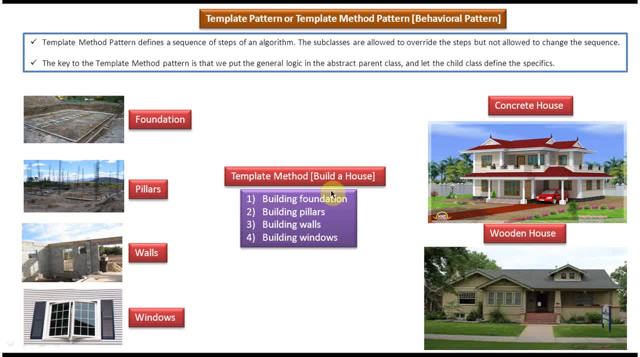 can define some kind of template method called build a house. so the template method defines what and all procedures I have to follow in order to build a house like step 1 is building a foundation, step 2 is building pillars, step 3 is building walls, step 4 is building windows. so for both the houses like